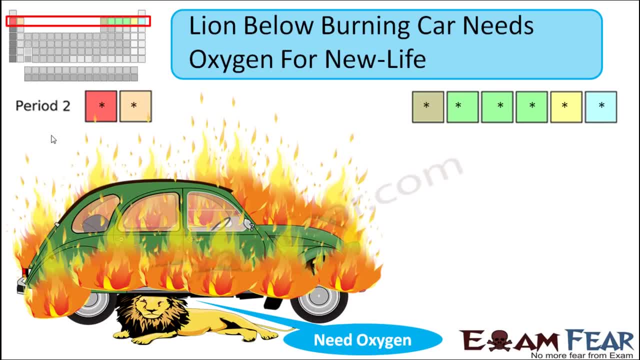 imagine that how the lion must be feeling right now. So the lion must be craving for life and it needs oxygen urgently, right? So the memory tip here is: lion below burning car needs oxygen for new life. So what does this reminds us of? So lion reminds of lithium Li in lion, Li in. 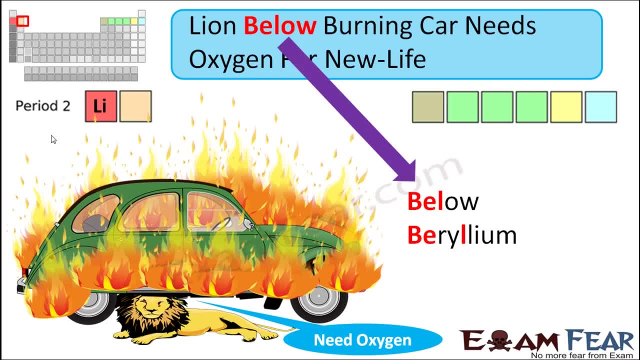 lithium, So lion reminds of lithium. Below reminds of beryllium, So be be So. below is beryllium Burning. reminds of boron, So burn boron, burn boron, So burning is boron. Car, of course, reminds. 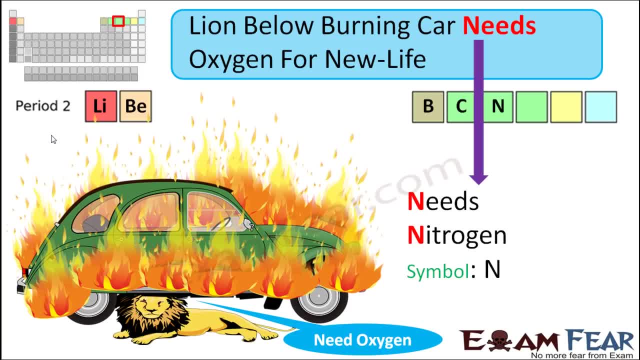 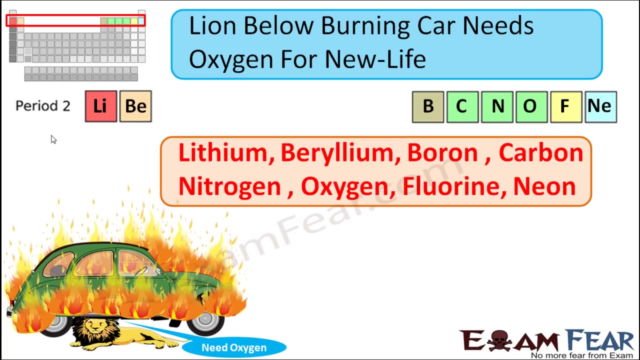 of carbon with symbol c Needs. Needs again N in nitrogen. So needs reminds of nitrogen. Oxygen, of course, is oxygen For reminds of fluorine And new life reminds of neon. So finally, our memory tip for elements in period 2 would be Lion below burning car Needs. 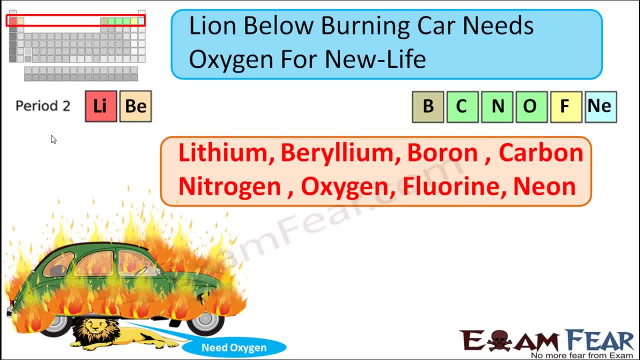 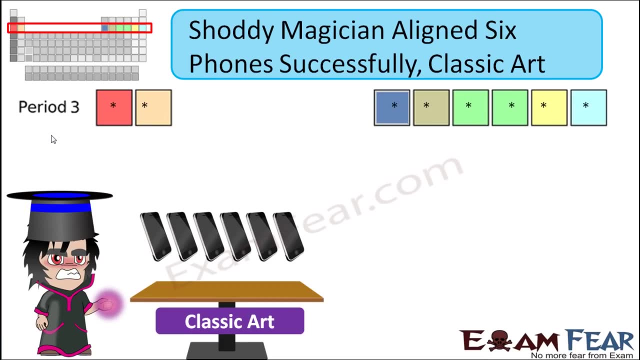 oxygen for new life. Now, if you just remember this picture, that's enough. So, remembering the picture, you will be able to remember the memory tip, and once you remember the memory tip, you very easily remember the name of the elements. Let's move on to period three. So what do you? 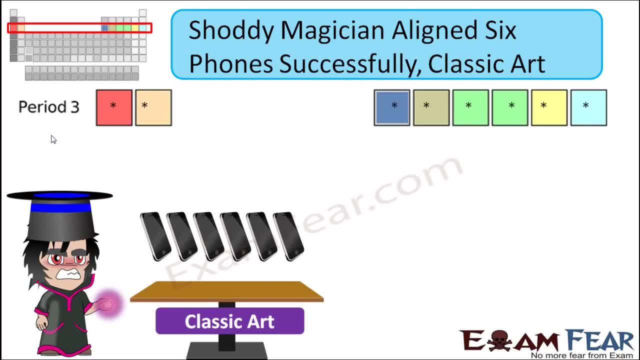 think is our memory tip, looking at the picture that we have on the screen. So we have a dirty magician who is doing some sort of magic with mobile phones and in fact we see that some six mobile phones have been kind of hanging in the air and that's his classic art. So the memory tip. 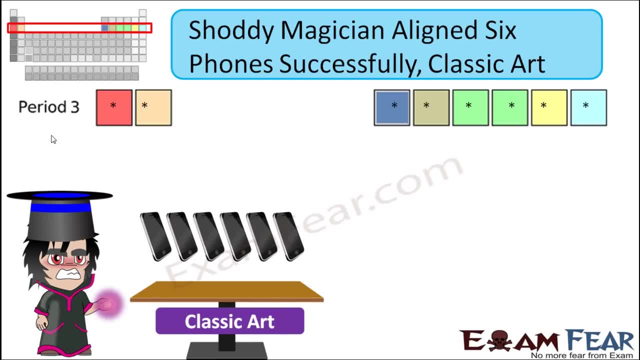 here is Saudi magician aligned six phones successfully- Classic art. So here Saudi. reminds of sodium with symbol N. A Magician reminds of magnesium, So mag in magician, mag in magnesium, So that's magnesium Aligned. reminds of aluminium Six. 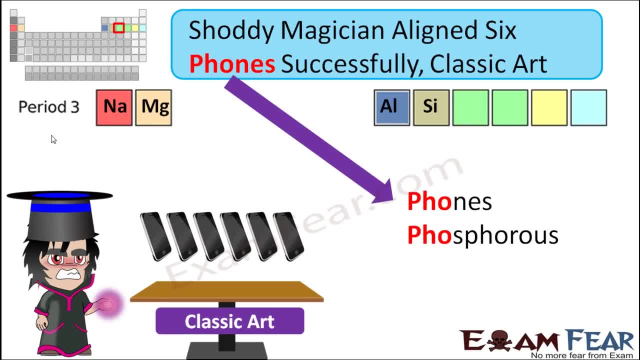 Six is silicon, So six silicon Phones. reminds of phosphorus Successfully. reminds of sulfur S U in successfully S U in sulfur, So successfully. reminds of sulfur Classic. reminds of chlorine, So chlorine classic. Similar Art. reminds of argon, So finally. 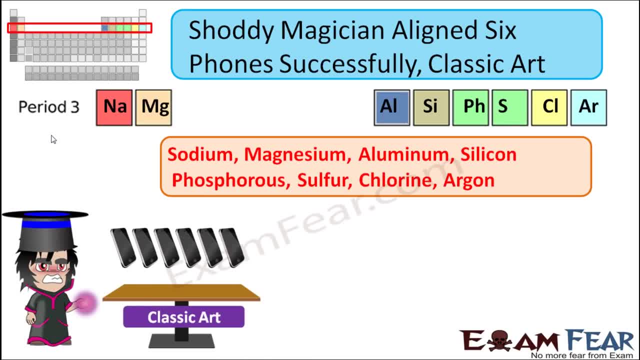 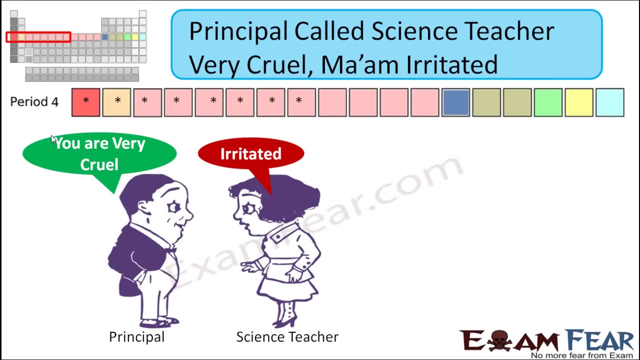 the memory tip for elements in period three would be sodium magnesium. So, finally, the memory tip for elements in period three would be: Saudi magician: align six phones successfully- Classic art. Moving on to period four, We see on the screen that there is a principal. 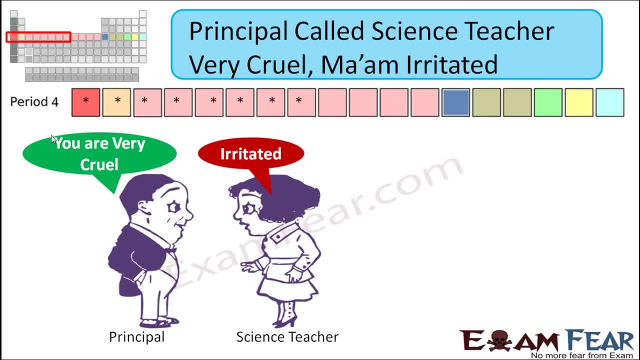 who is telling something to the science teacher and the teacher is getting really irritated. Now here, if you look at period four, there are huge number of elements here And there's a lot of elements here. Now, what do you think of all the elements here, in these three elements here? 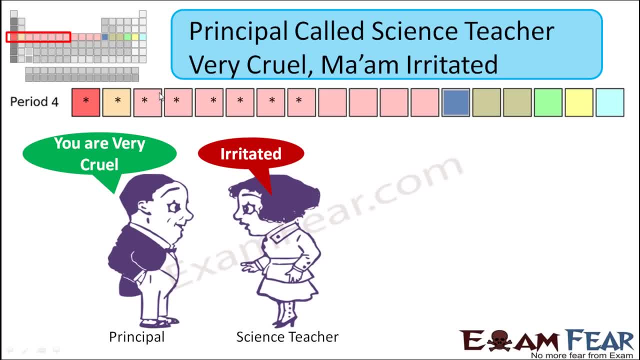 There are a lot of elements here, But then they are not so much but more of a combination, The elements in period four, and that is why we have divided it into two sections. so right now we will only discuss about the first section. so looking at the picture, you see that the memory tip for 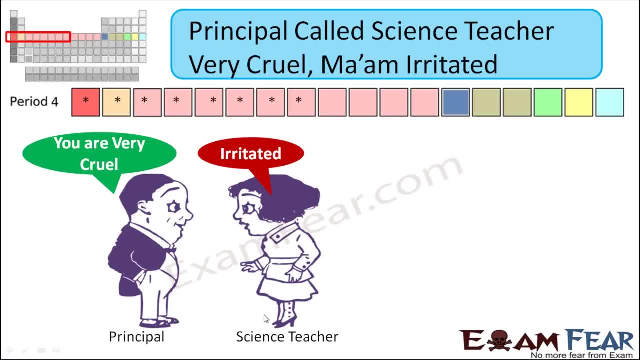 period four would be principal called science teacher. very cruel, ma'am irritated. so here principal reminds of potassium, p in principle, p in potassium. however, the symbol for potassium is k, so please remember that. so principal reminds of potassium, called reminds of calcium. so you have Cal in, called again Cal in calcium, so called reminds of calcium. science reminds of scandia. 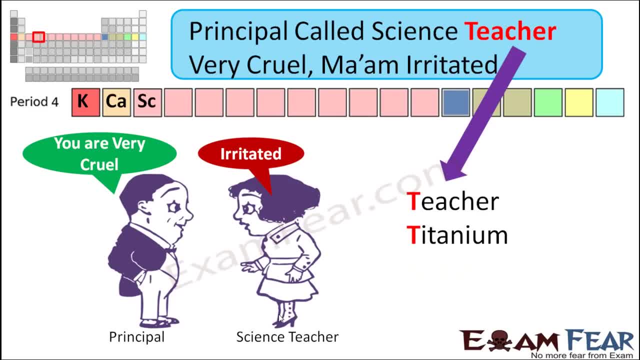 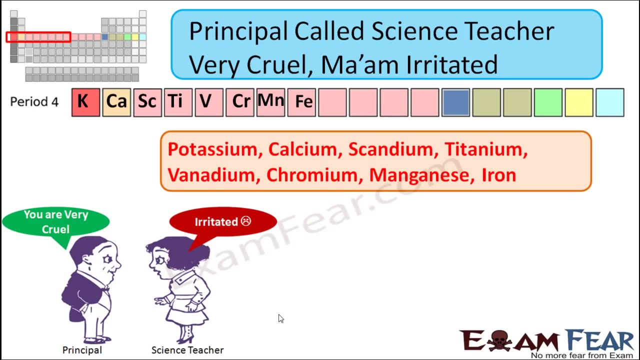 with symbol SC teacher reminds of titanium, very reminds of vanadium. cruel reminds of chromium. so you have crawl and cruel. crawl in chromium, so cruel chromium. ma'am reminds of manganese and irritated reminds of iron. so ir in irritated, ir in iron. however, the symbol for iron is fe. so what's our final memory tip for the first half of period? four elements. 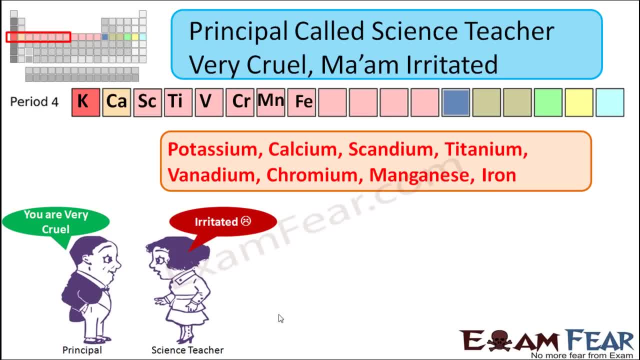 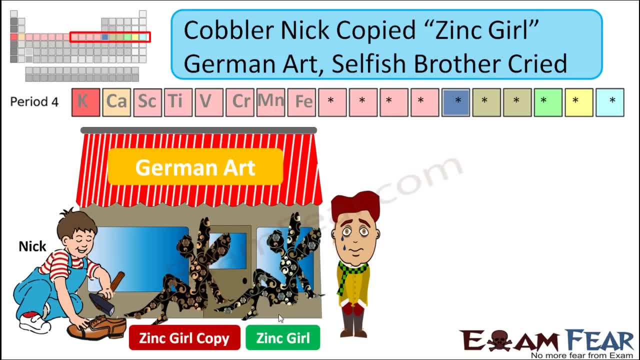 that's principal, called science teacher. very cruel, ma'am irritated. let's move on to the next half of period four. she research area. so Билар сказал: к gardens. so the story, the construction of there is a proper ma'am وال, there is a. 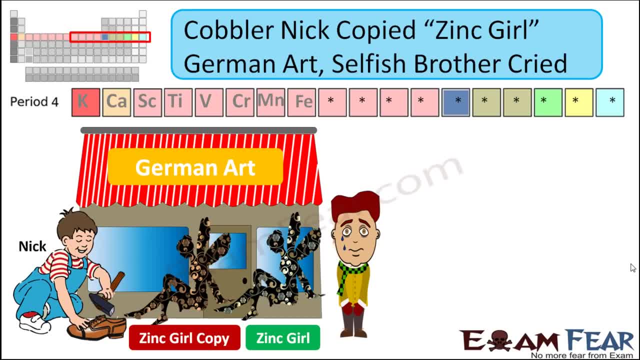 by the cup art gallery. okay, so here. cobbler reminds of cobalt, nick nickel copied. reminds of copper, zinc is, of course, zinc. girl reminds of gallium, german germanium art. reminds of arsenic, with symbol as and not ar. ar is argon, so arsenic is as selfish. reminds of selenium, so cell in selfish. 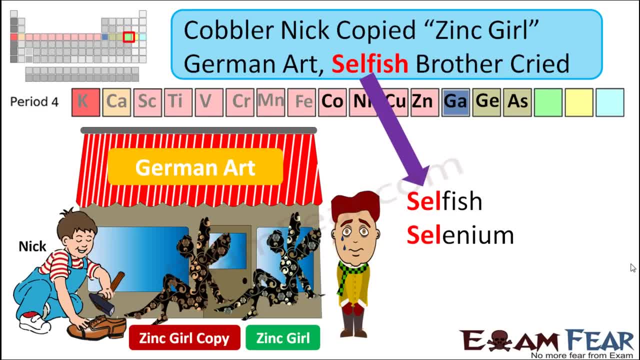 cell in selenium, so selfish, reminds of selenium. brother reminds of bromine, so you have a bro and brother, you have a bro in bromine. and finally, cried reminds of krypton. so here just focus on the pronunciation. so in cried, you have cra in krypton. you have cra, so cried. 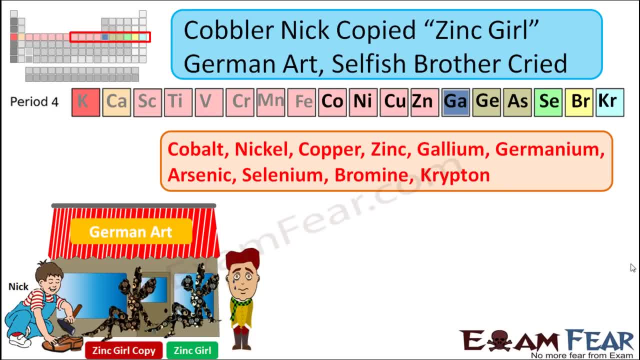 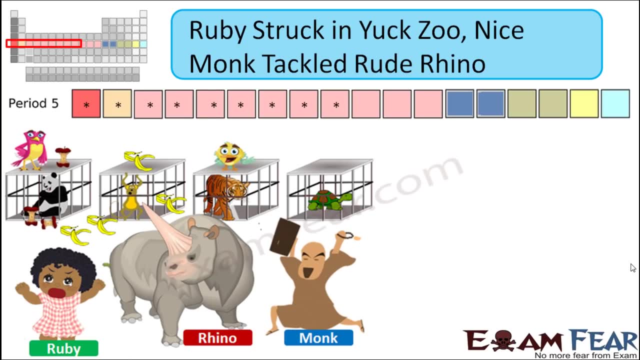 krypton. so finally, the memory tip for the elements in the second half of period four is: cobbler nick copied zinc girl german art selfish brother cried. moving on to period five, again, we have divided period five into two halves, so right now we will focus only on the first half. so what do? 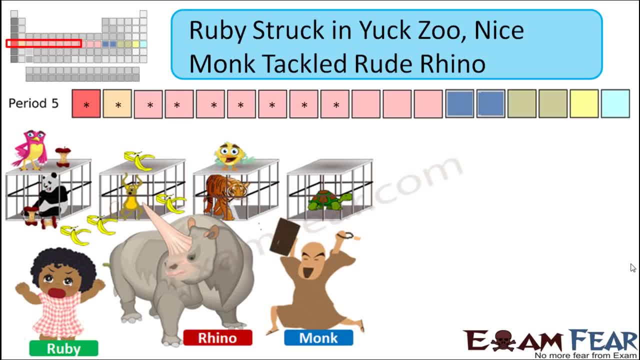 we see here. so we see that it's a zoo where we have a lot of animals, but at the same time there are a lot of dirt and dust littered around, so it's kind of a dirty zoo. we see a big and dangerous rhino. we also see a little girl named ruby and also a monk. so the story here is this. 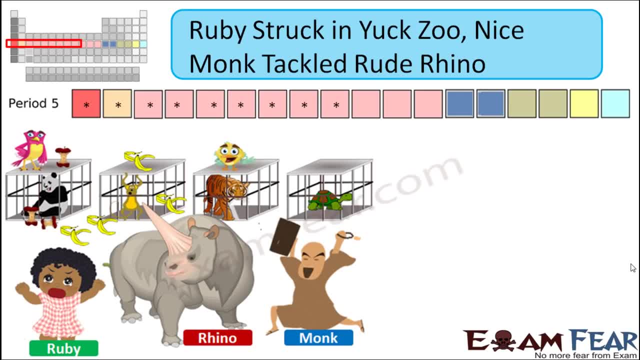 little girl was stuck in this dirty zoo and the monk comes and he, he somehow handles and tackles this big rhino. so our memory tip would be: ruby struck in yuck zoo nice trois. so this is yuck zoo. the story is that when they implement a new letter like ruby's truck in yuck zoo, they add five jerks. so when the car was parked for the parking garage. the car was parked and the car was parked. so the positions immediately follow that if it is the wrong address will be the same that růby's truck in yuck zoo, and then the close而且 this is the probably. 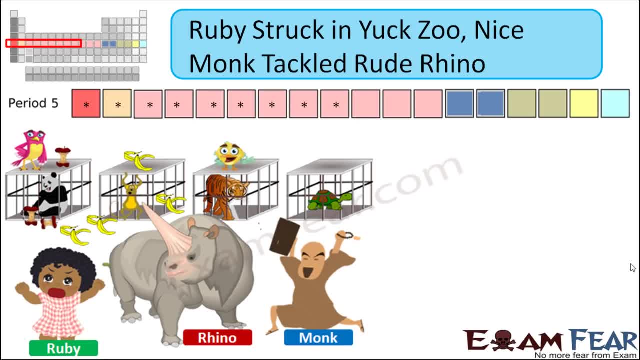 yakzu. nice monk tackled the rude rhino. So ruby reminds of rubidium, struck reminds of strontium, yak reminds of uterium, with symbol y zu reminds of zirconium. nice is niobium, monk is molybdenum, tackled is technetium, rude is rudenium and finally, rhino is rhodium. 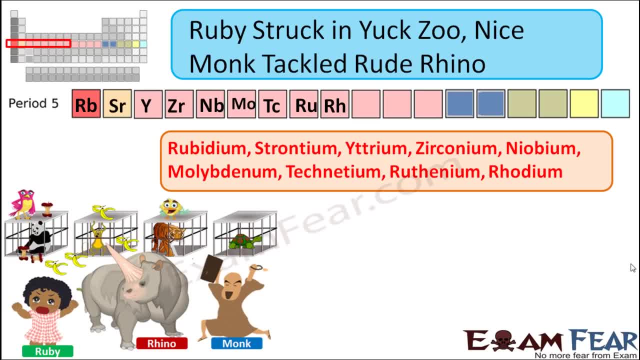 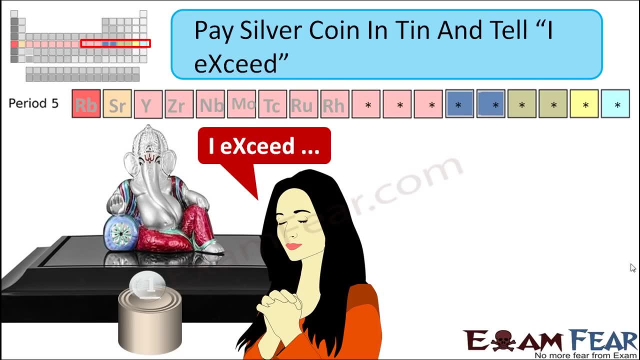 So our final memory tip for the elements of first half of period 5 would be: ruby struck in yakzu nice monk tackled rude rhino. Moving on to the second half of period 5.. Here we see a good, good girl praying. In fact, we also see that the girl is not only praying in front of the God. 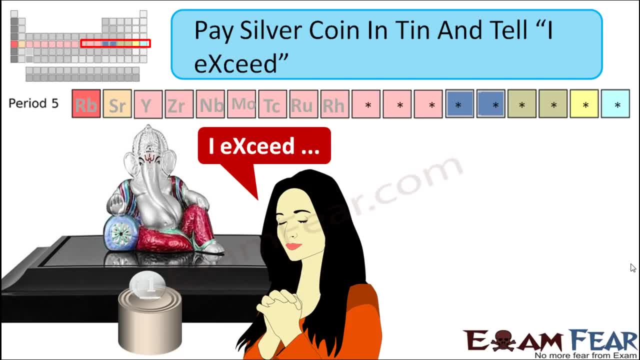 but looks like that she has put a coin into the tin container and she's telling that I exceed. I think this is a very common scenario for all of you during exam time. When you go, you visit temples, you pray to God that okay, I put a one rupee coin for you, but please get me good score. 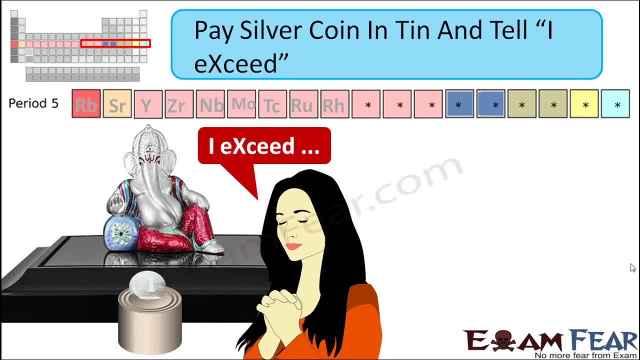 in exam. So that's a very common scenario which you can relate to. So here your memory tip would be: pay silver coin in tin and tell I exceed. So here, pay reminds of palladium. silver is, of course silver. however, the symbol for silver is A G Coin reminds of cadmium in reminds of indium. tin is tin again. 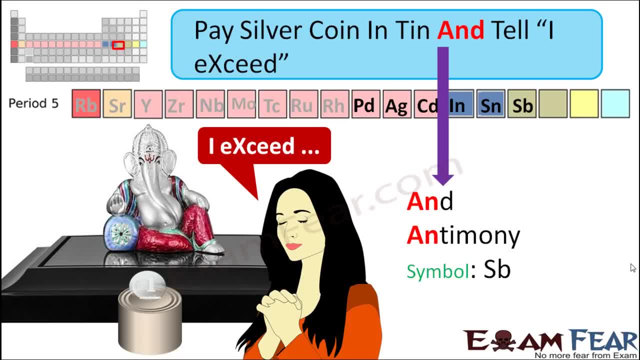 and is antimony, So you have an in and you also have an in antimony. So it's- and reminds us of antimony And in antimony. you also have an in antimony, So it's an in antimony, So it's an in antimony. 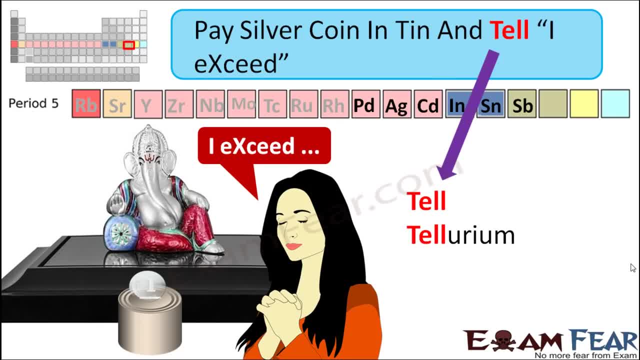 but the symbol for antimony is SB. TEL reminds of tellurium, I reminds of iodine, and XSEED reminds of xenon, with symbol XE. So basically, when you look at XSEED, so it reminds you of XE and XE. 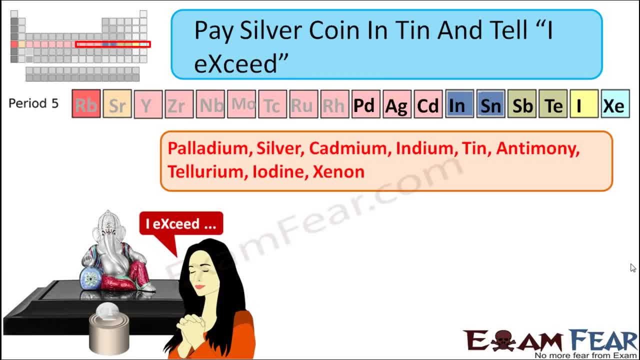 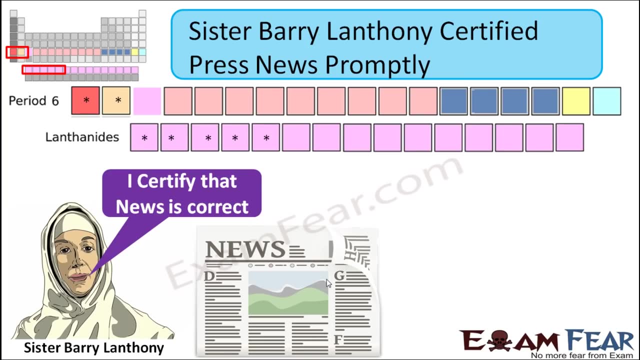 is the symbol of xenon. So our memory tip for second half of period 5 would be: pay silver coin in team and tell I XSEED. Let's now look at period 6.. Now in period 6, we have huge number. 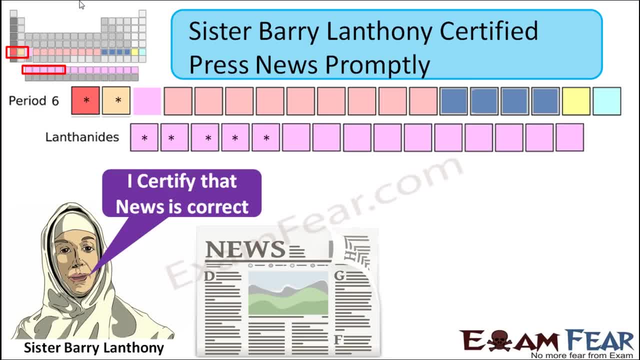 of elements. In fact, we have a total of 32 elements in period 6.. So if you look at period 6, here it includes the entire lanthanide series. Like, this is the first element of period 6,. second element and the third block that you see, the pink block, it represents the entire lanthanide. 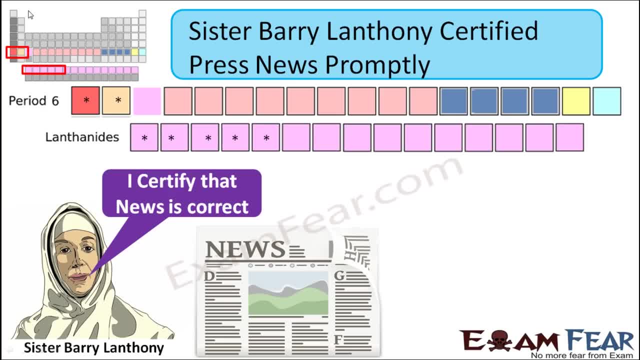 series. So right now we will focus on the first two elements and first five elements of the lanthanide series. Now let's look at the picture that we have here. So we have the picture of sister Barry Lanthony and she is telling that I certified that the news is correct. So the memory tip for us would 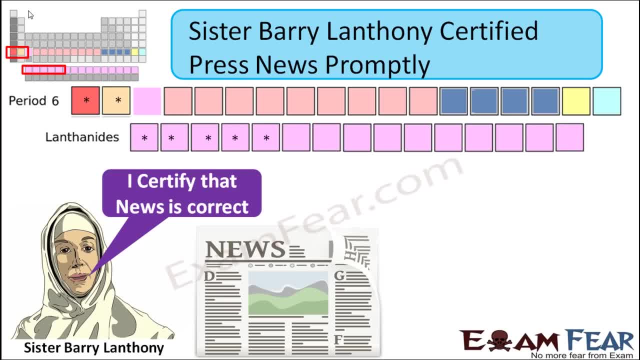 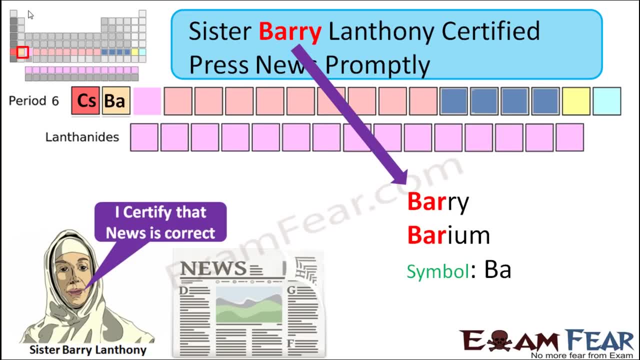 be sister Barry Lanthony certified press news promptly, So here, sister reminds of cesium with symbol CS. Barry reminds of B Barium with symbol B. Lans vuel reminds of Lanthenum. Certified for cerium. Press for prisodumium. News for neodymium. 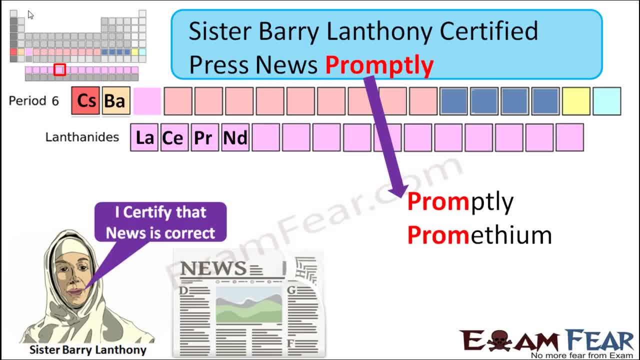 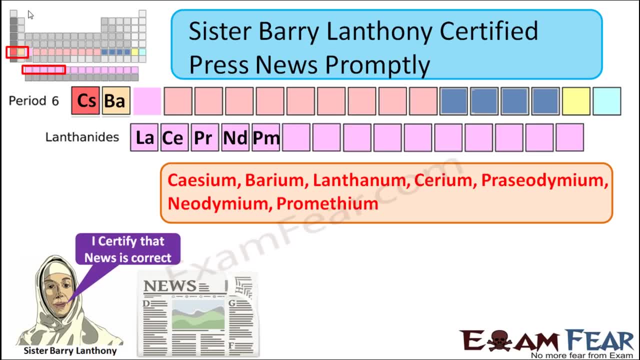 and promptly for promethium. So our final tip for this first two elements of period 6 would be: sister Barry Lanthony: certified press news promptly Now. another interesting thing There is: Now Lanthony reminds us that the lanthanide series starts from here, because the first element of 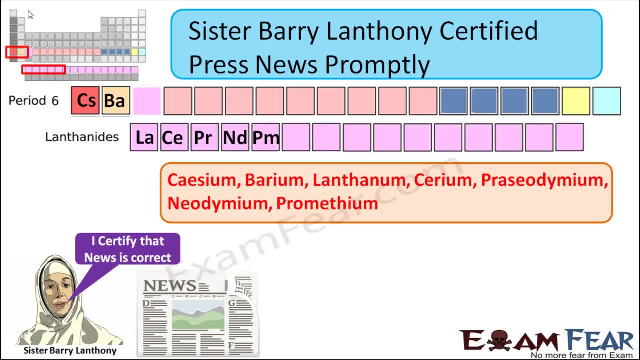 the lanthanide series is lanthanum, So lanthony is for lanthanum. So wherever you have lanthony, that is the beginning of the lanthanide series. So the lanthanide series starts with lanthanum, followed by cerium, praseodymium, neodymium, promethium and so on. 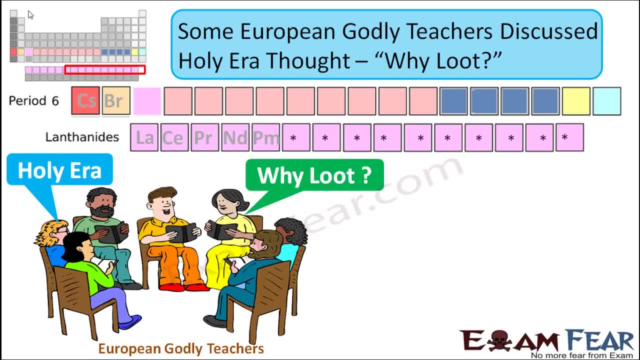 Now let's move on to the rest of the elements of lanthanide series. So what do we see on the screen? We see a group of teachers and they are discussing something. So they are discussing that today, in today's world, it's corruption all around. So there is no peace: corruption and 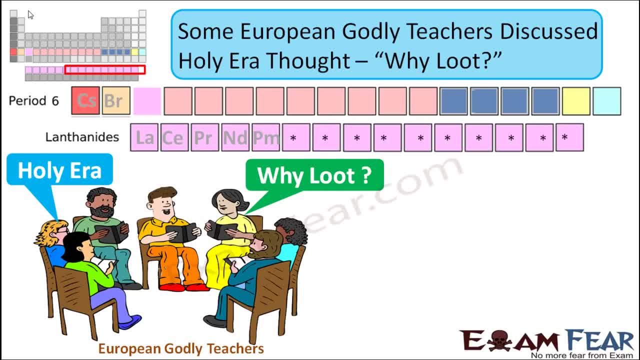 corruption everywhere. Now they are reading some holy era books and are saying that there was no loot during those times. There used to be no loot during those times. So they are saying that there was no corruption, no loot and it used to be peace all around. So they are saying that. 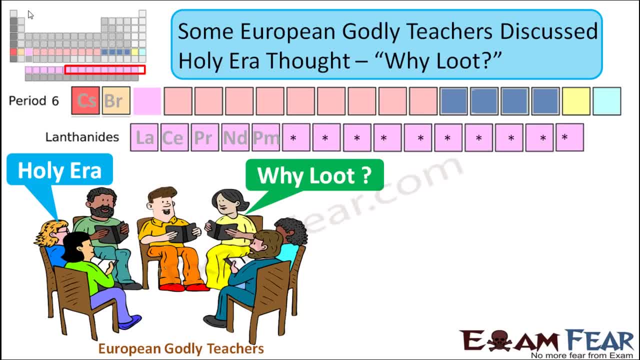 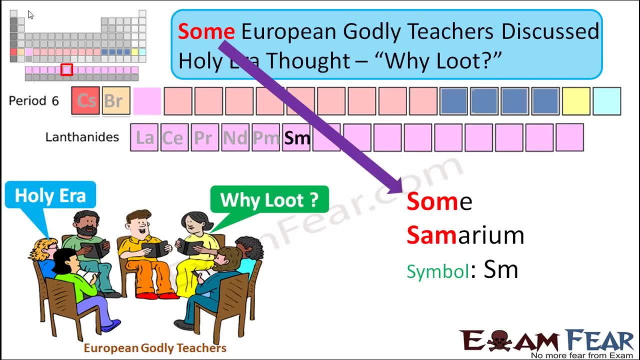 so, remembering that holy era thought, they are asking each other that why loot today? So the memory tip. here is some European godly. teachers discussed holy era thought: Why loot? So here some reminds of samarium with symbol sm. European reminds of europium, Godly for gadolinium Teachers. 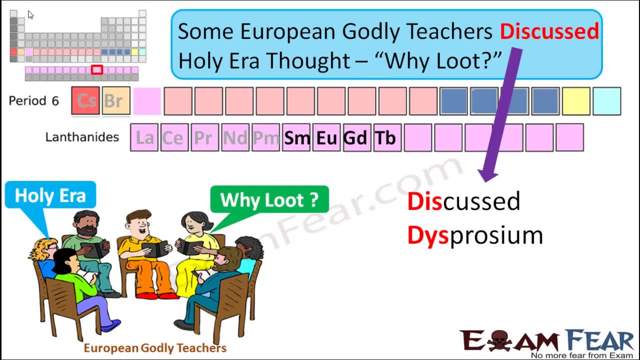 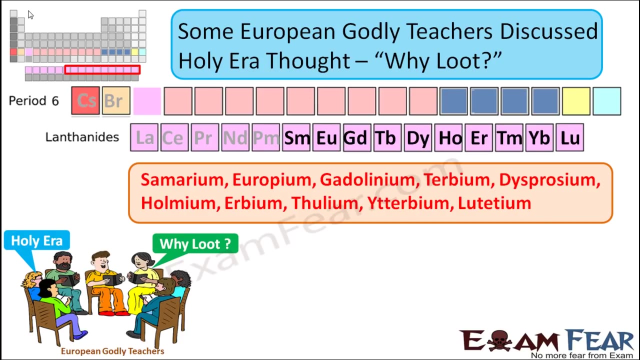 for terbium, Discussed for dysprosium, Holy for holmium Era for erbium, Thought for thulium. Why for eterbium with symbol yb And loot for lutetium. So our memory tip for the next set or the final. 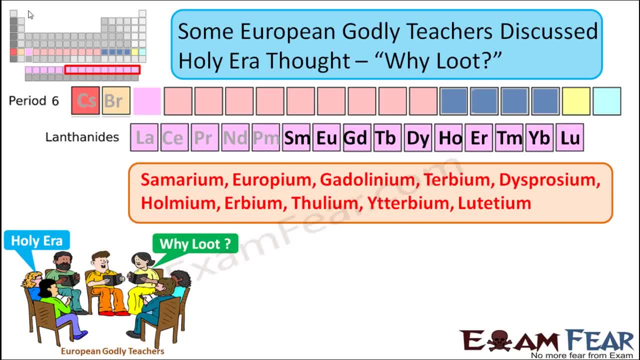 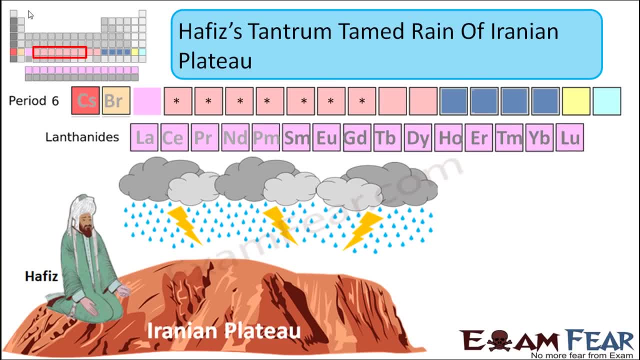 set of the lanthanide series would be. some European godly teachers discussed holy era, So they are saying that holy era thought, Why loot? Now let's move on to the next set of elements for period six. So here we see a saint named Hafiz who is sitting at the Iranian plateau and he is trying. 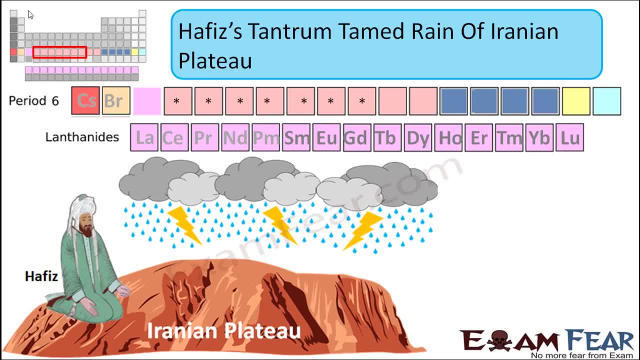 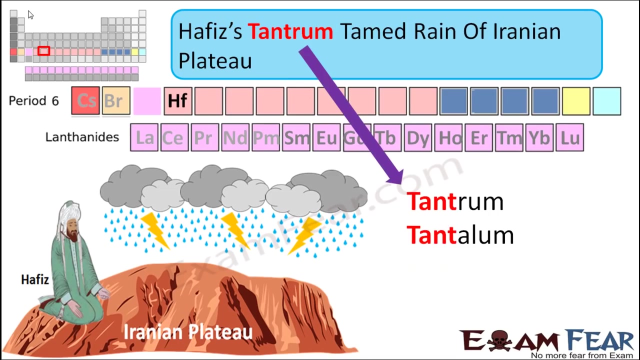 to control the rains with his tantrums. So our memory tip here is Hafiz tantrum, tamed rain of Iranian plateau. Now let's move on to the next set of elements for period six. So here we see a saint on the attorneys table. So here has a young man in white. tamed rain of phobes. Now his Night back is the date of firstylon, of Budhohana, Otherwise a hermitage. So first rite of the sun or the Capricorn, And then, in his death, of the senate. So here is. 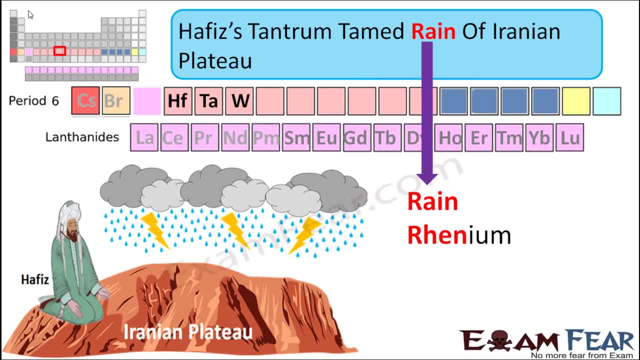 T and its tungsten. The symbol is W: Rain for rhenium, off for osmium, iranian for iridium. So IR in iranian, IR in iridium. So that's how they match. Plateau for platino, So that's PT. 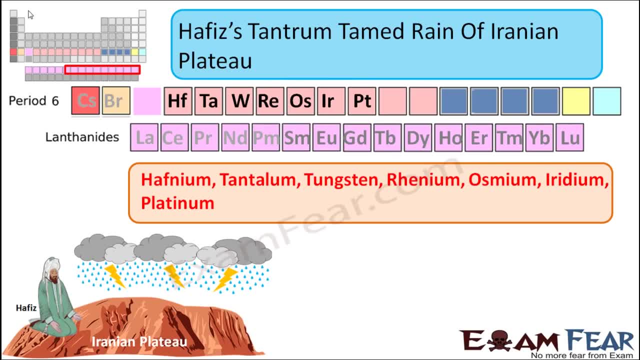 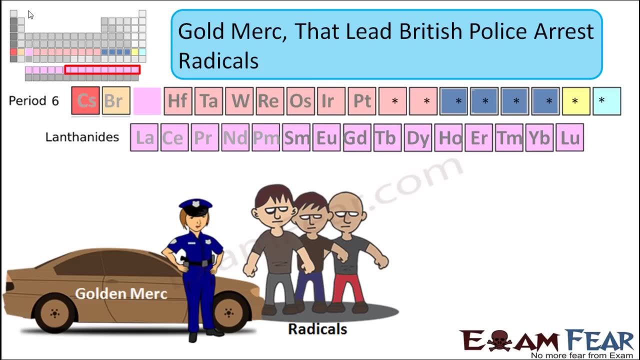 So, finally, the memory tip for this set of elements of period 6 would be Hafiz tantrum, tamed rain of iranian plateau. Finally, the last set of elements of period 6.. We see on the screen a golden Mercedes and a police who is arresting the radicals. 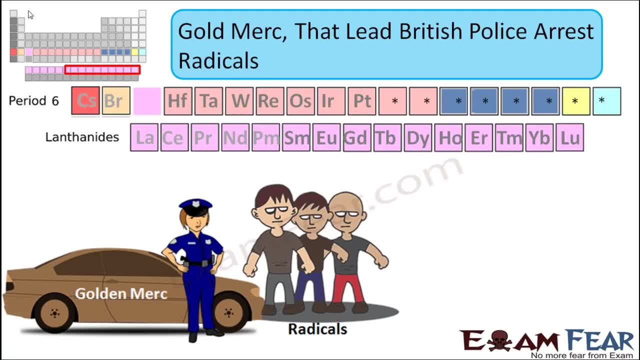 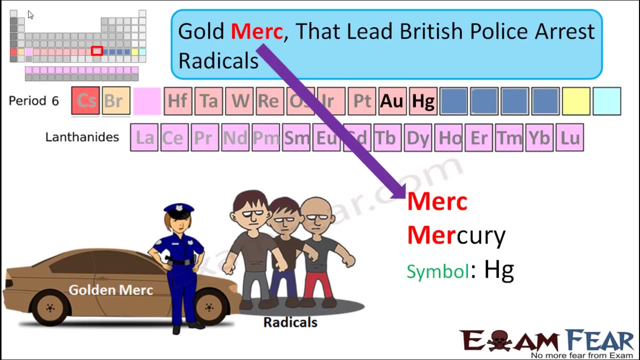 2-3 radicals, which are people with some kind of negative thought in the society. So the memory tip here would be gold mark that led British police arrest radicals. So gold is of course gold. Merck reminds of mercury, with symbol HG That reminds of thallium. 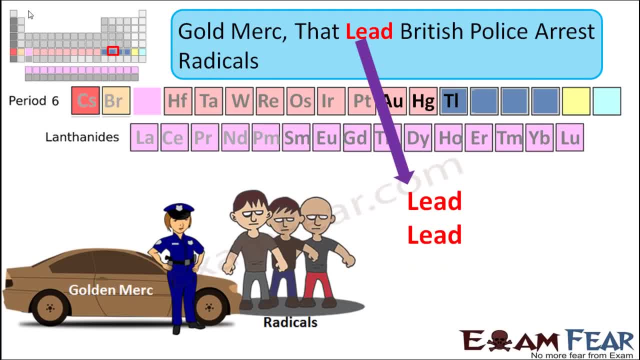 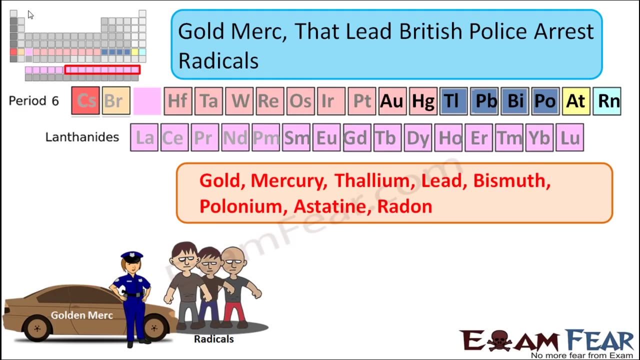 with symbol TL. Lead is again lead. British reminds of bismuth with symbol DI. Police reminds of polonium with symbol PO, Arrest reminds of astatine And radicals reminds of radon. So our memory tip for this last set of elements of period 6 would be gold merck that led British. 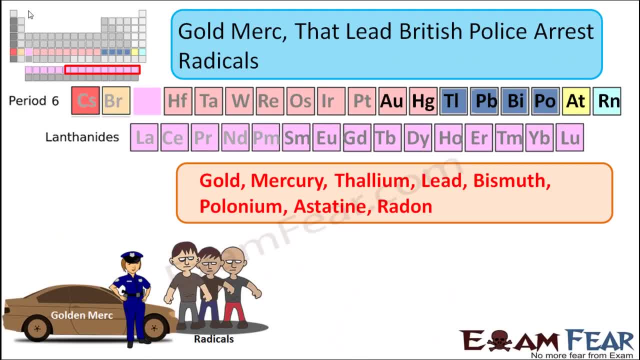 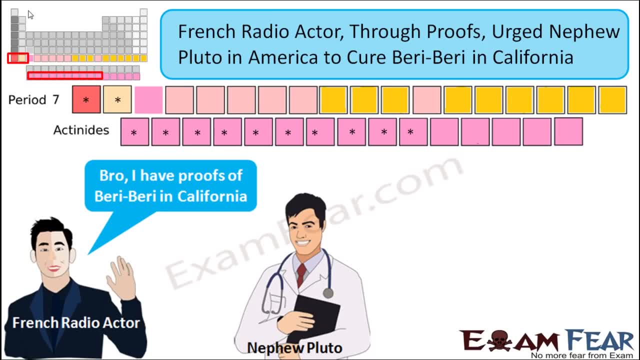 police arrest radicals. Now let's move on to period 7.. And here we see a French radio actor who is telling that, Bro, I've proof of beriberi in California and he is trying to inform his nephew named Pluto, who lives in America. 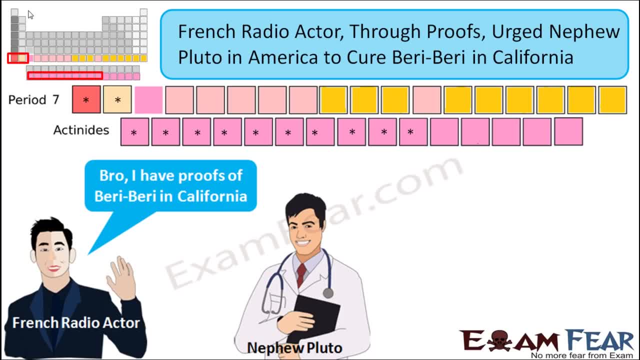 So is french radio. actor through proves, urged nephew pluto in america to cure beriberi in california. so here, french reminds of francium, with symbol fr, radio reminds of radium. actor for actinium, through for thorium, proves for protactinium, urged for uranium. nephew for neptunium, pluto is. 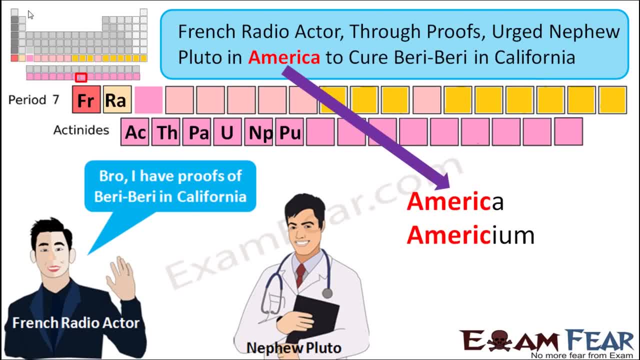 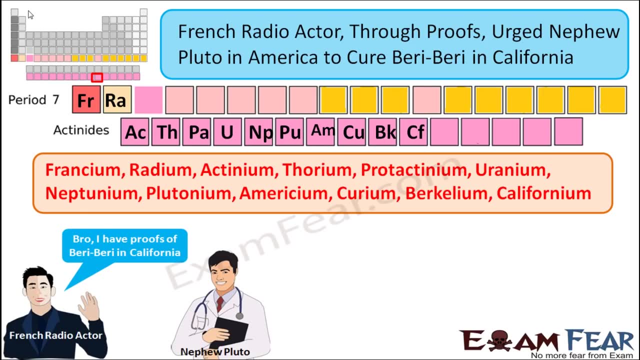 plutonium. america is americium, cure is curium, beriberi is berkelium and california is californium. so our final memory tip for the elements of period 7 would be francium radium. so these are the elements and the memory tip would be: french radio actor: through proves urged nephew pluto in america. 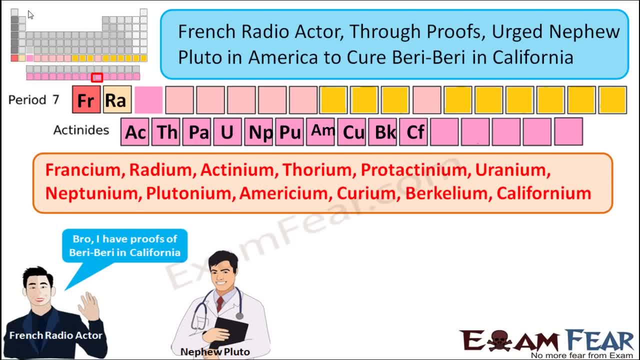 to cure beriberi in california. so in period 7 as well we have a total of 32 elements and inside this period 7 we have the actinide series. so the element actinium is. it marks the beginning of the actinide series. 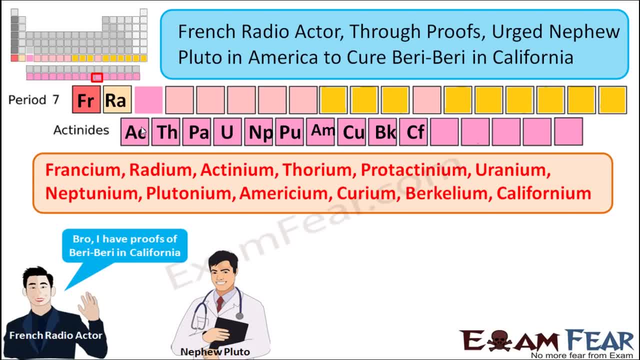 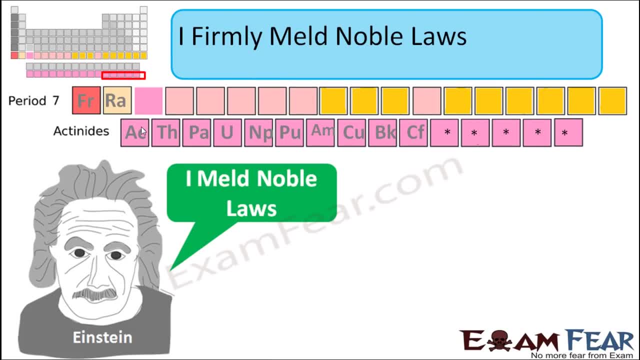 so when you have actor, actor reminds you of actinium and actinium tells you that the actinide series have begun. now let's move on to the second half of the actinide series. so we see here this word: i is an actinide relationship process. 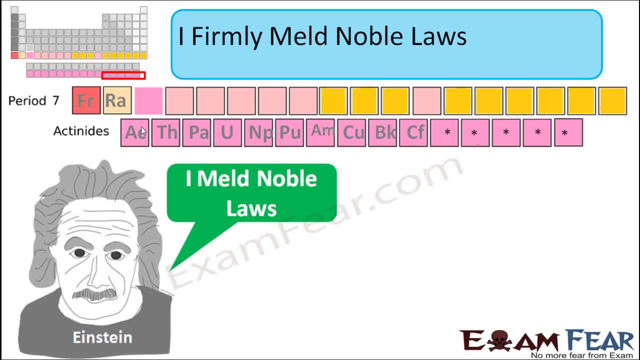 and what case? y bloom is a people here is ai name was a science icon, but i here is called the. trying to Firmly is for fermium, melt is for mendelevium, noble is for nobelium and loss is for laurentium. 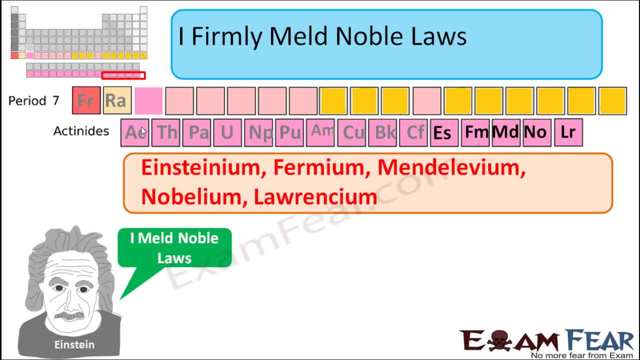 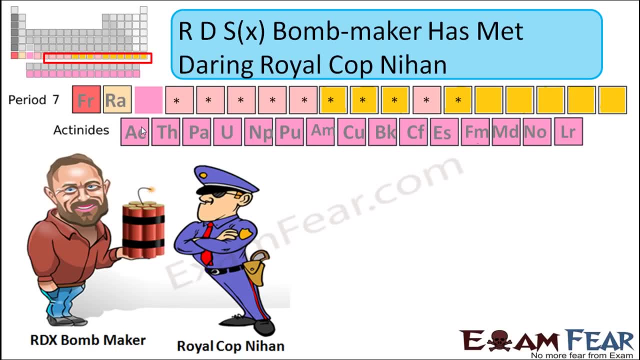 So our memory tip would be: I firmly melt, noble loss. Now let's move on to the remaining elements of period 7.. So what do you see on the screen? We see a RDX bomb maker and he has kind of, you know, faced or he has been encountered by the royal cop named Nihan. 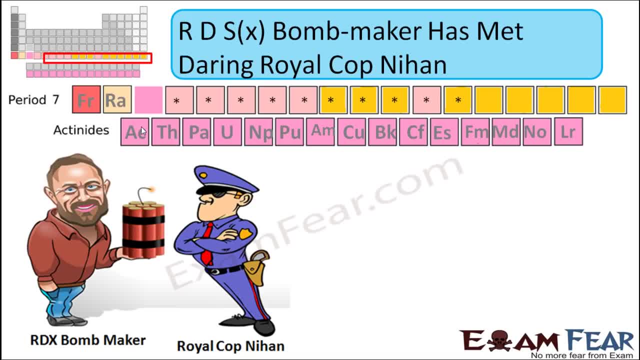 So our tip here is: RDX bomb maker has met daring royal cop Nihan. Here R reminds of rhodophodium, with symbol RF D for dubnium, with symbol DB S for sibogium. Bomb maker reminds of boron. 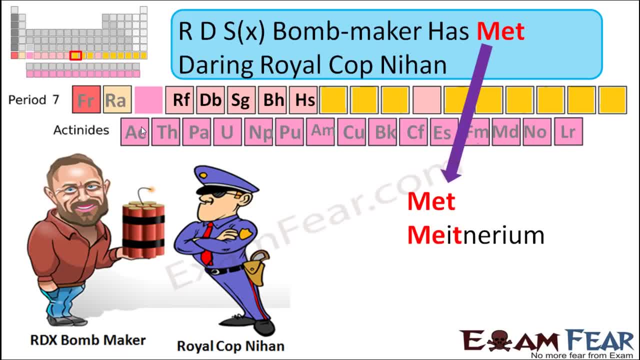 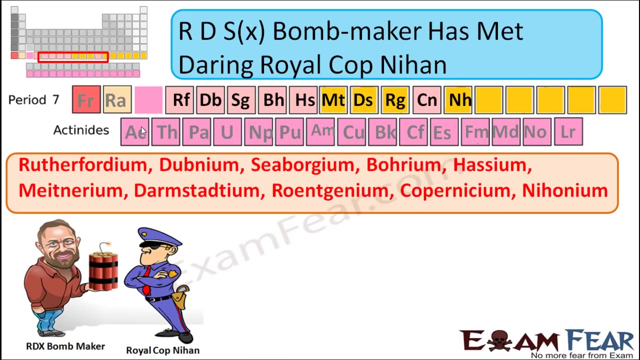 Has for hasium, met for meturnium, daring for damstuadium, royal for roentgenium, cop for copernicum and Nihan for nihonium. So our final memory tip for these remaining elements of period 7 would be: 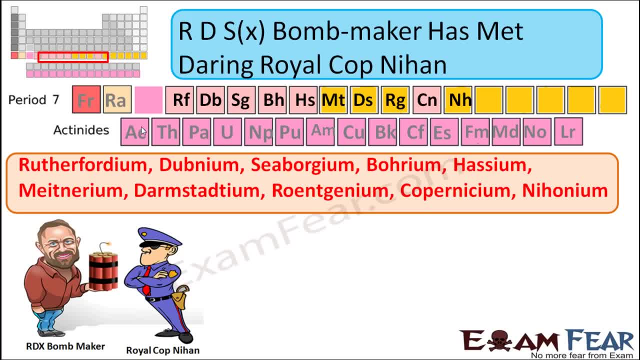 RDX bomb maker has met for nobelium, has for hasium, met for meturnium, daring for damstuadium, royal for roentgenium, cop for copernicum and Nihan for nihonium, whereas on RDX, bomb maker has met daring royal cop nihan. 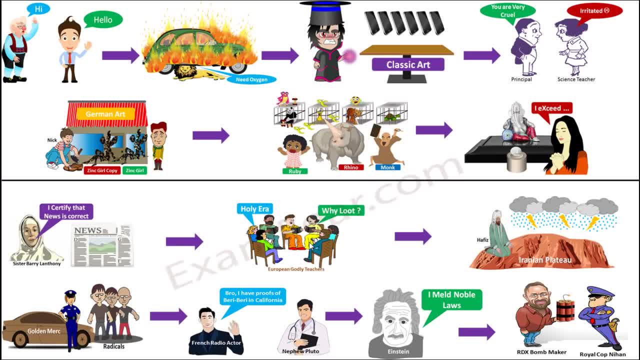 Now, if you remember each memory type on each storyline, you would be definitely able to remember the elements of that particular period. But now the question is: how can we remember the sequence of these storylines? So for that, we have one single story which will help you to remind the sequence of the storyline. 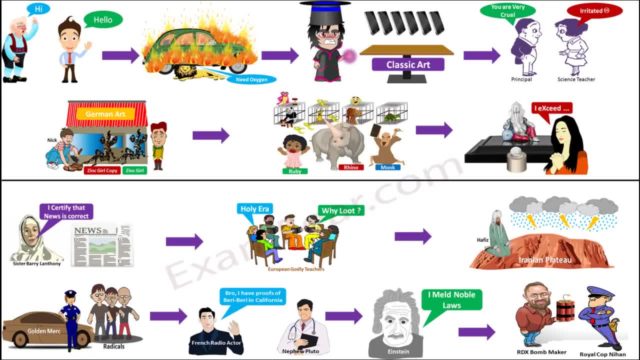 So this story is about how you start your day. So you start your day day. your grandfather wishes you hi and you reply him hello, and that's how your day starts. then you take up your car, which reminds you of the storyline of the burning car. you take your car and go to a 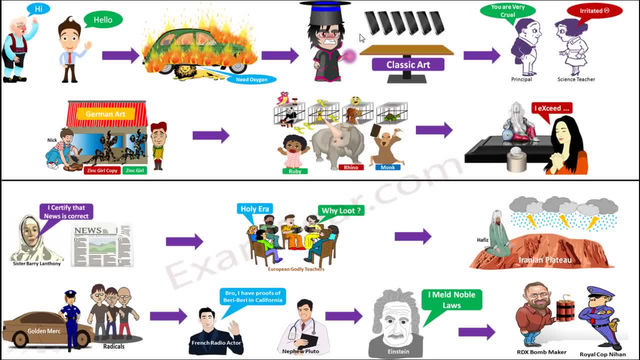 magic show which again reminds you of the magician, the Saudi magician, who was doing some magics with the phone. now, after attending the magic show, it's your time to go to your school. so you go to your school and there you see that your science teacher was told by the principal that she was very cruel. 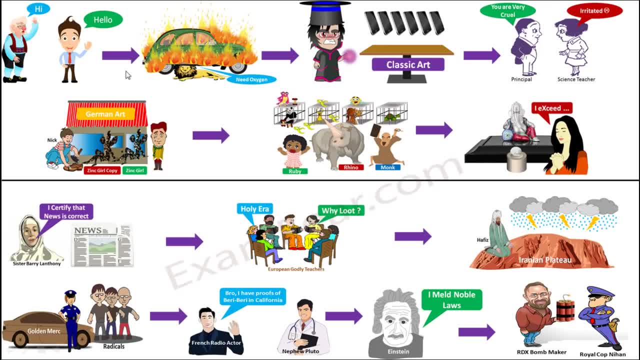 which made her irritated. now, once you're done with your school, while coming back home, just outside your school, you have your cobbler friend, Nick. so and that day Nick was very happy because he was able to copy the famous zinc girl, German art. so he was very happy and to celebrate his happiness. 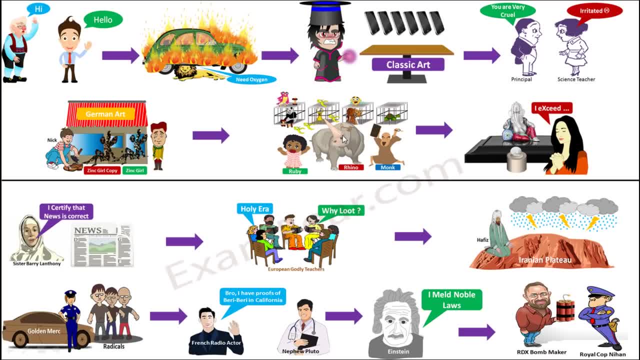 you, along with Nick, went to the zoo and fortunately the zoo was very dirty and yucky and you- you were some somehow trapped there, but then a nice monk came and saved you both. so after coming back from the zoo you went to the temple and you thanked the Lord that you know you were very kind of saved from the zoo and you are safe. 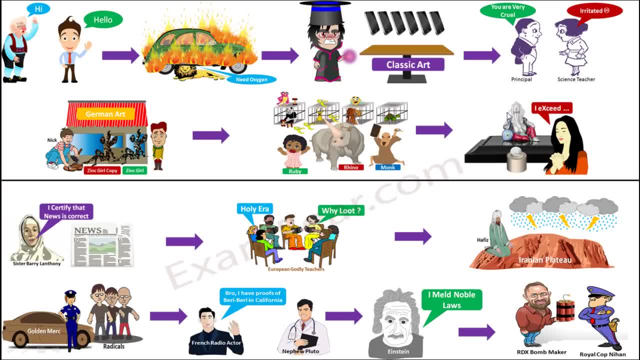 so you thanked the Lord. so this, when you thank the Lord, this reminds you of the memory tip where we, the other kids, say the crop could have been put into a church, and that's the thing which says that you pay a coin in the tin and you tell: 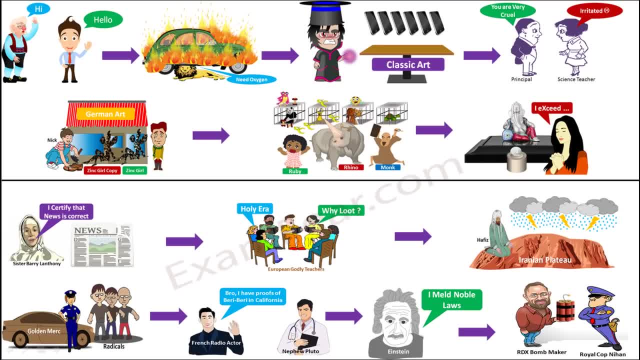 that I exceed and you are done. so you are done for the day. so you come home, you sleep for the day. when you wake up next day morning it's time for Newspaper. so when you open the newspaper to have a look at the headlines, you see that sister Barry lanthony has finally certified each other. the news is correct and this news is basically about the loot and so sister barrylanthsiy has finally certified that the news is correct and this news is basically about the loot and all the bad things, алf, the bad things that's happening. so material laisser is form氯x or faity that. 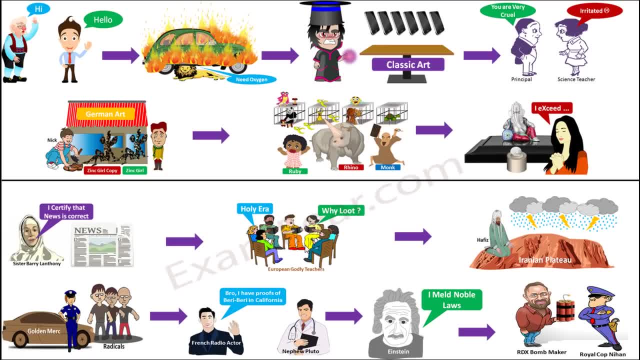 the loot and the all the bad things that's happening around us. so there is a lot of discussion happening regarding why this loot, why so much of loot everywhere around, and it was found that one of the causes of this loot is the lack of rain or drought, which has happened in Iran. now, besides that, in the 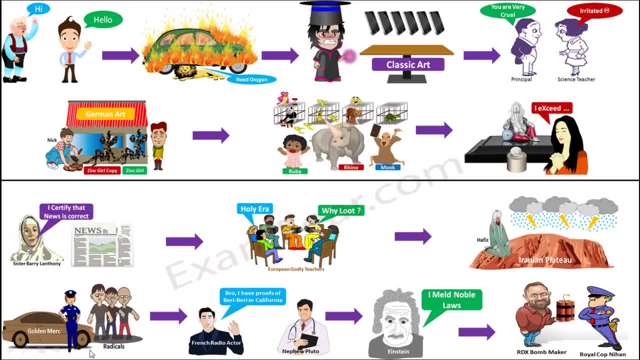 international section of the newspaper you also saw that the British police police could actually arrest the radicals who were involved in the golden Mercedes case. and you also found that in America there is this dr Pluto who would be working to find out a cure for beriberi in America. so after having a 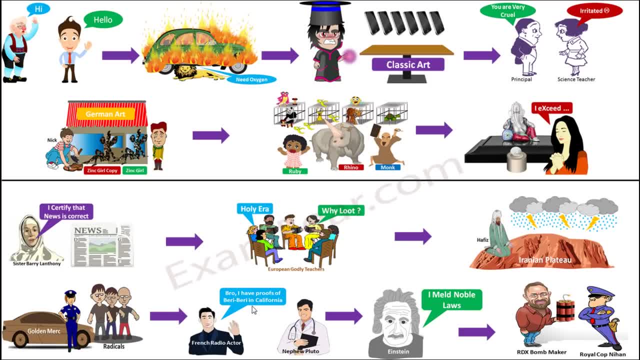 look at all the news which were there, all the important news in the newspaper. it's your time to sit for study. so you set for study and you open your physics book because it's your physics exam today. and you have, you start studying the Einstein's laws in physics now, after a 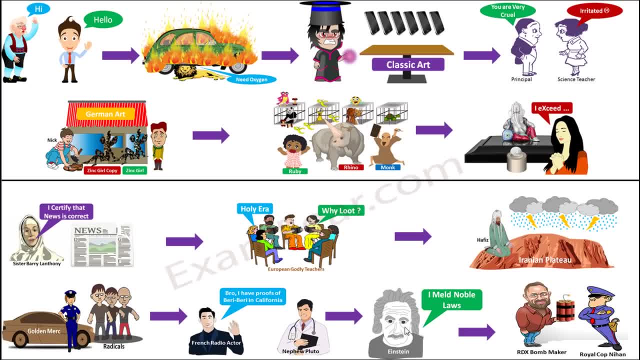 couple of minutes of study, you suddenly start feeling quite sleepy and, you know, drowsy and you actually slept off while studying. now, when you slept off, you actually saw this dream where you found that you- so we assume that your name is Nihon. so in the dream you actually saw that you are the royal cop Nihon, who. 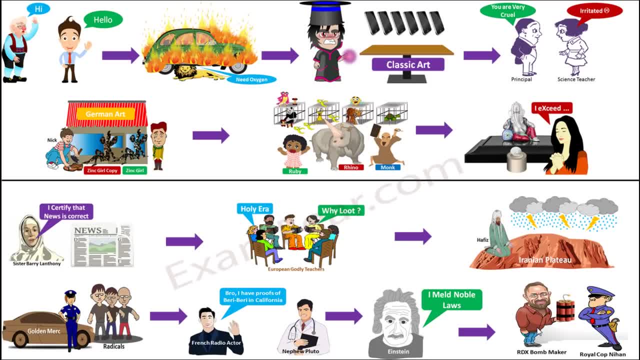 actually arrested the RDX bomb maker, so that that was like a very- you know, interesting and a very nice dream which made you feel very happy and enthusiastic. so I think, with this story lines, this story line will help you to remember the sequence of the story lines or the sequence of the memory tips. 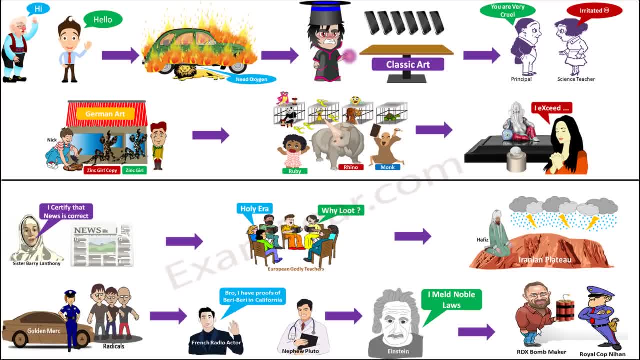 because remembering the sequence of memory tips is very important. only then you will be able to remember the sequence of the elements in the order of their atomic number. so I hope that this strategy of making use of pictures to remember the elements of the periodic table will will be useful to you. so make.